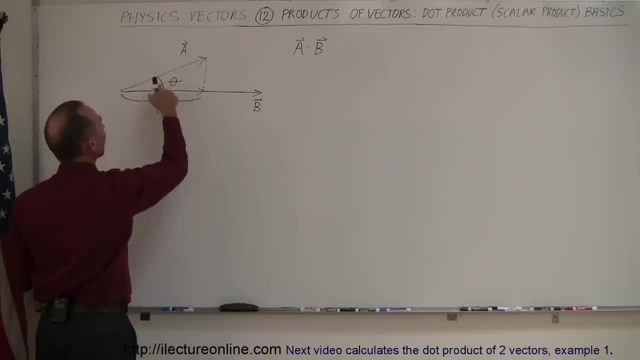 the vector a, which is the hypotenuse of this triangle, Times the cosine of this angle, theta. So this distance, here the magnitude, is a times the cosine of theta. So now it turns out that a dot b or a multiplied by b via the dot product, is equal to: 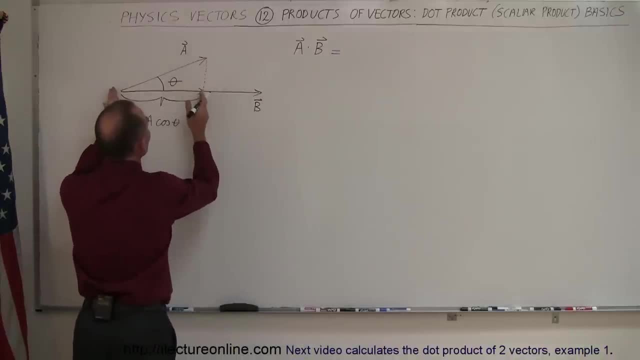 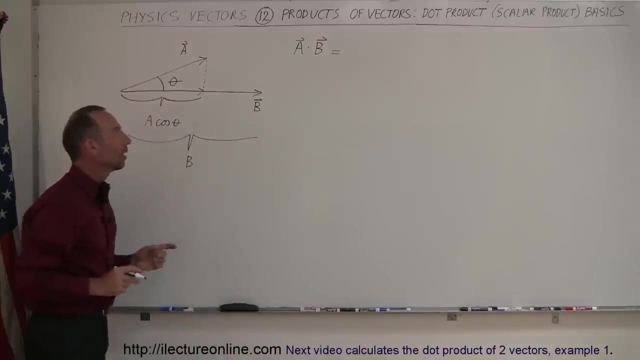 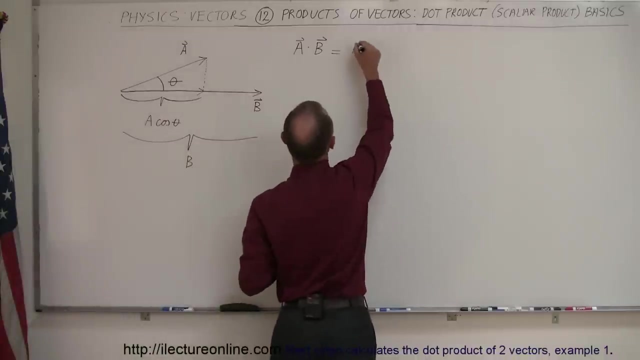 the length of the projection of this vector onto the b vector times the length of the b vector. So if I go ahead and realize that this is the magnitude or the length of the b vector, the dot product is simply The distance or this length times this length. So what that means, it is equal to a times the cosine. 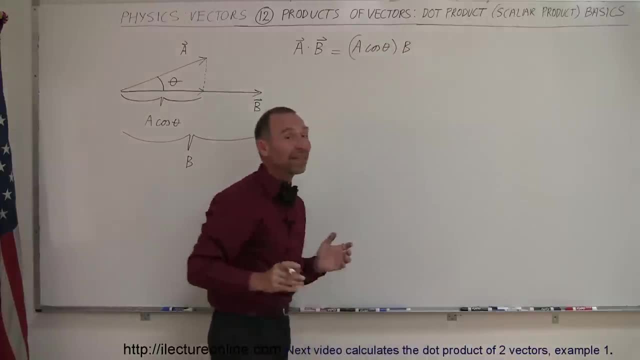 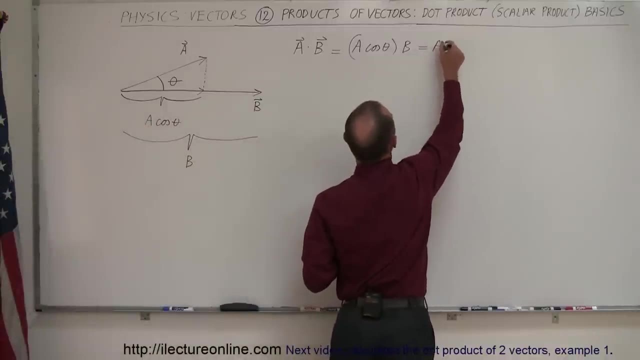 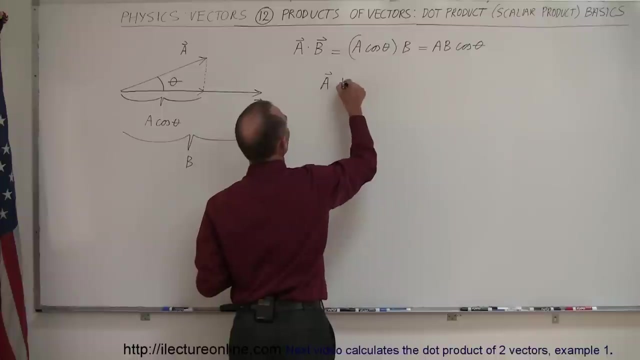 of theta times b. So that's, by definition, the dot product. Now we usually write it like that, We usually write it like this: This is equal to a times b times the cosine of the angle between them. So, again written in a more compact fashion, a dot b is defined as a times b times the cosine of theta. 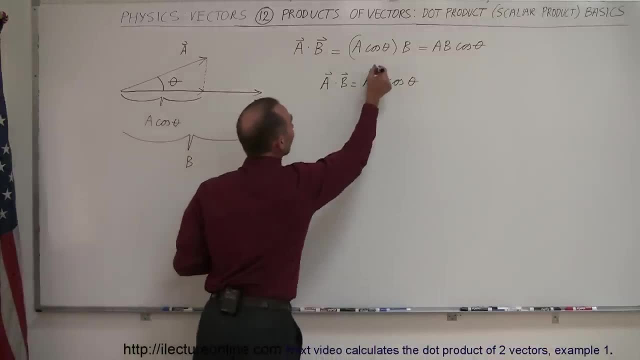 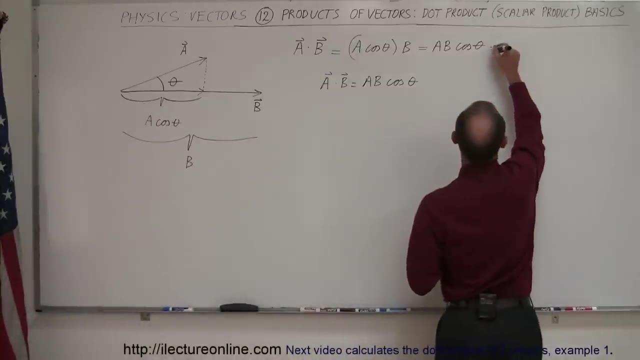 Now remember that a and b, without the little lines on top, means the magnitude of a and the magnitude of b. So really, what we could have done is we could have written it like this: This is equal to the magnitude of a times the magnitude of b, times the cosine of theta. 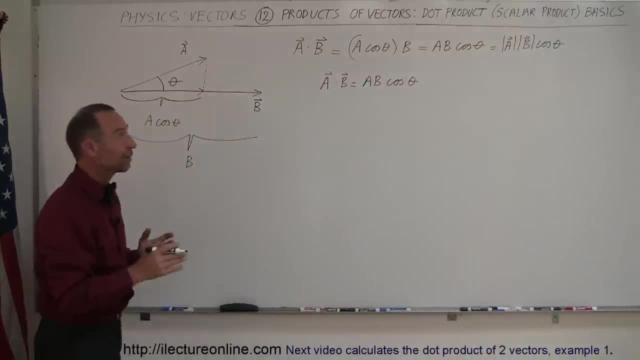 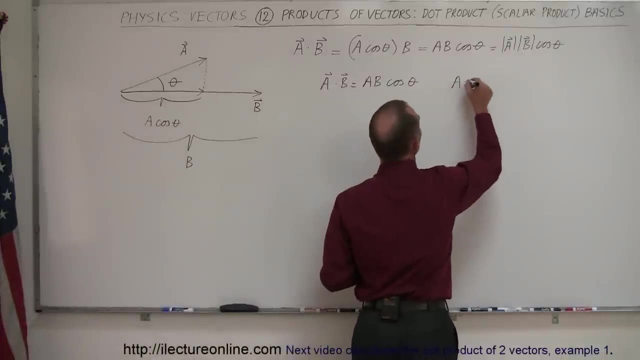 So just don't forget that a and b, without the little line on top, is simply the magnitude of those vectors. And you remember how to get the magnitude of the vectors? Well, the magnitude of a is equal to the square root of the x component of the. 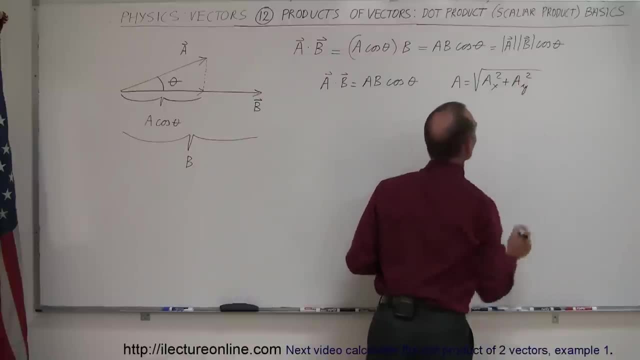 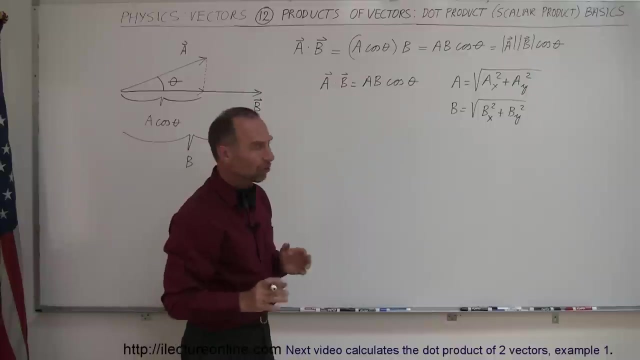 a squared plus the y component of a squared, and of course that's in two dimensions and for the vector b, that is equal to the square root of the x component of b squared plus the y component of b squared, And of course add them together and take the square root. Three dimensions, of course. this. 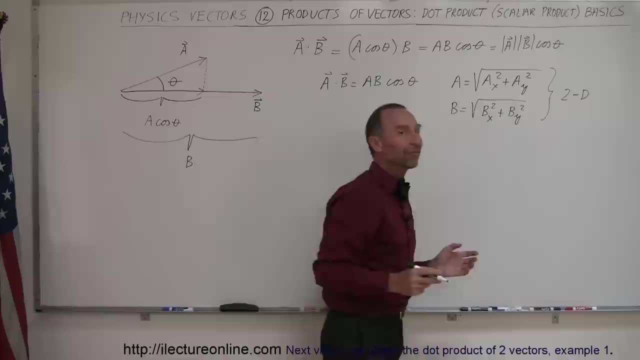 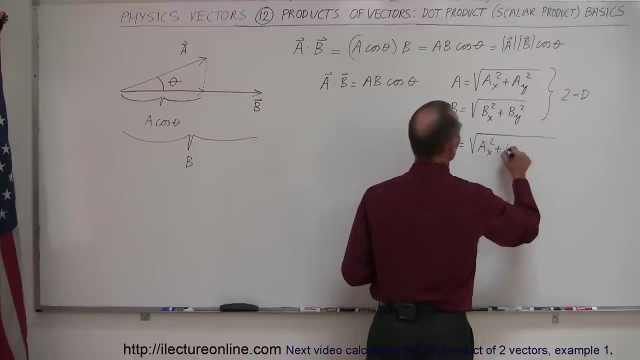 is in 2d or two dimensions. Of course. if we have three dimensional vectors, then the magnitude of a would simply be the square root of the x component squared plus b, the y component squared plus the z component squared added together and take the square root. 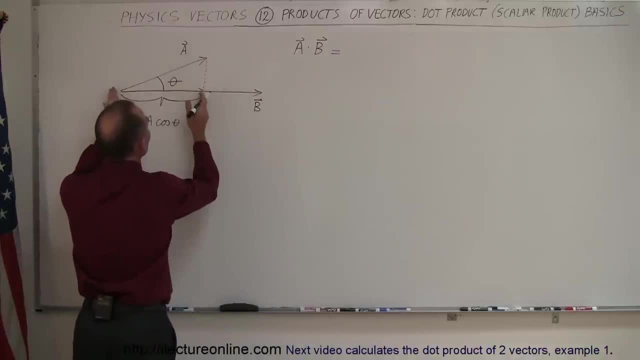 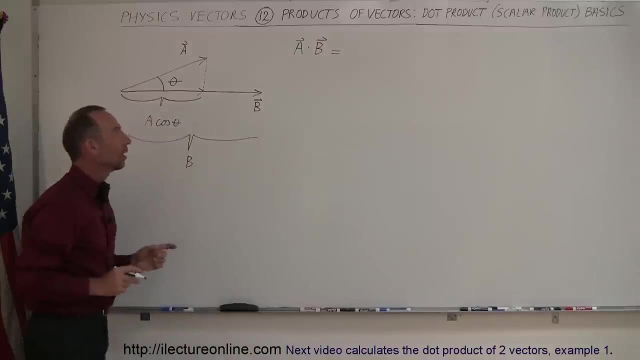 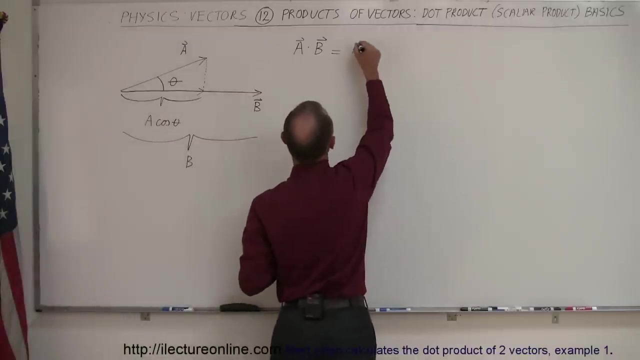 the length of the projection of this vector onto the b vector times the length of the b vector. So if I go ahead and realize that this is the magnitude or the length of the b vector, the dot product is simply this or this length times this length. So what that means is equal to A times the cosine of theta times B. 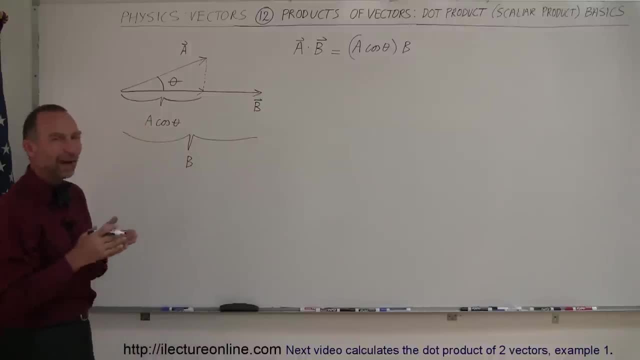 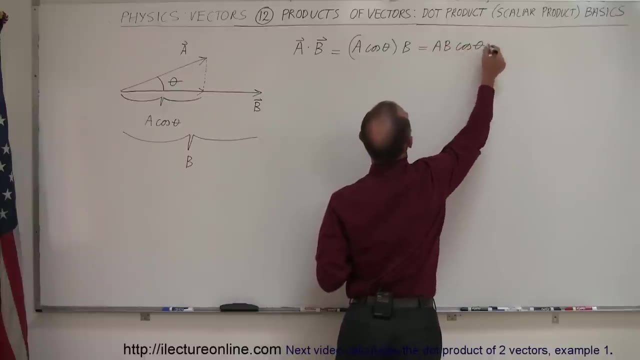 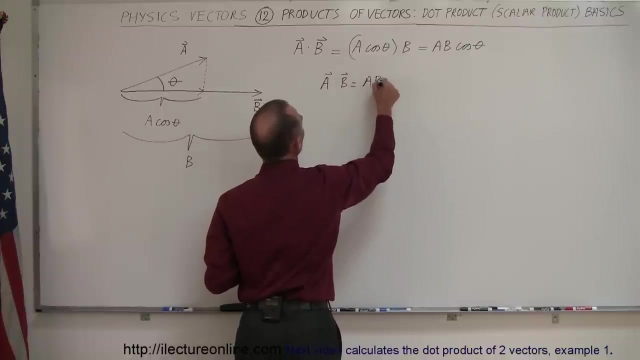 So that's, by definition, the dot product. Now, we usually don't write it like that, we usually write it like this: This is equal to A times B times the cosine of the angle between them. So, again written in a more compact fashion, A dot B is defined as A times B times the cosine of theta. 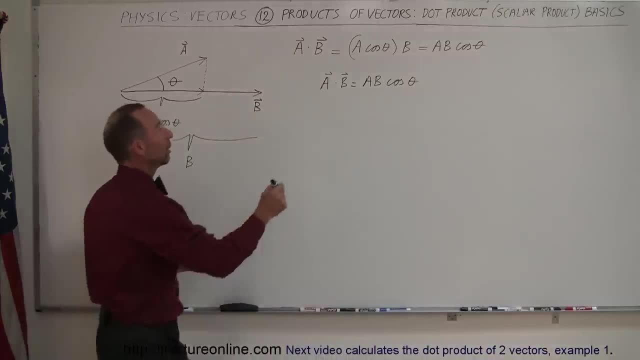 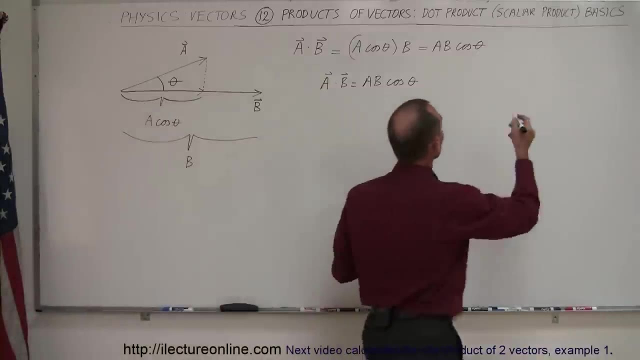 Now remember that A and B, without the little lines on top, means the magnitude of A and the magnitude of B. So really, what we could have done is we could have written it like this: This is equal to the magnitude of A times the magnitude of B, times the cosine of theta. 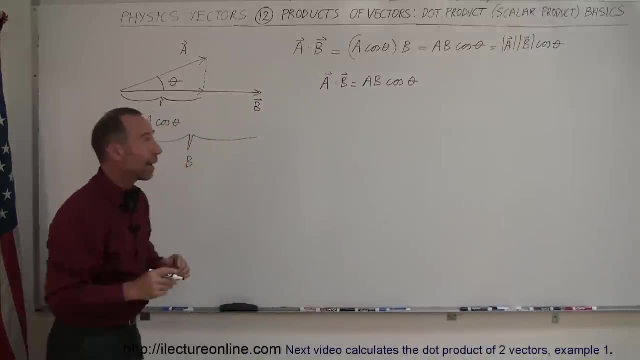 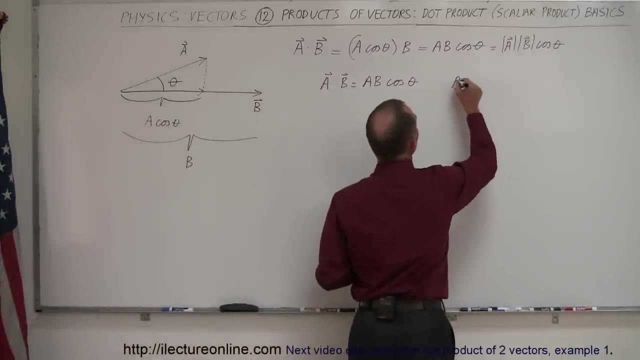 So just don't forget that A and B, without the little line on top, is simply the magnitude of those vectors. And do you remember how to get the magnitude of the vectors? Well, the magnitude of A is equal to the square root of the angle between them. 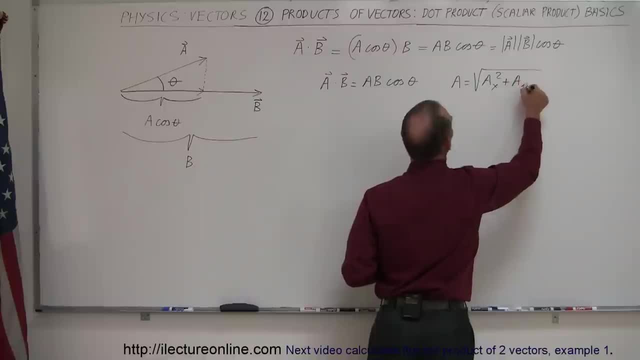 That's the x component of A squared plus the y component of A squared, And of course that's in two dimensions And for the vector B, that is equal to the square root of the x component of B squared plus the y component of B squared. 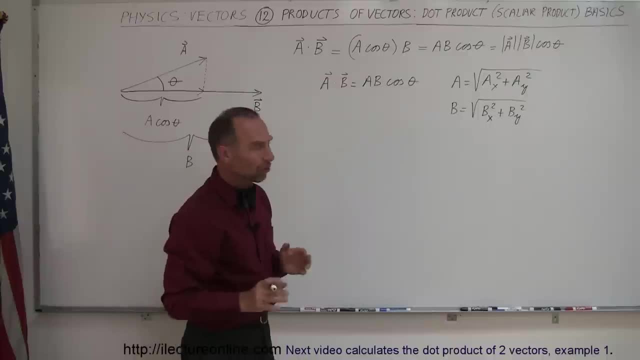 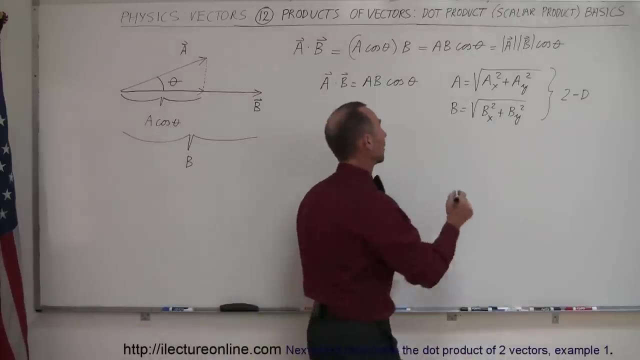 And, of course, add them together and take the square root In three dimensions. of course, this is in 2D or two dimensions. Of course, if we have three dimensional vectors, then the magnitude of A would simply be the square root of the x component. 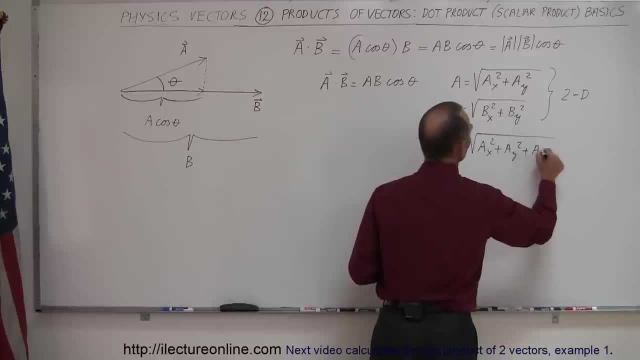 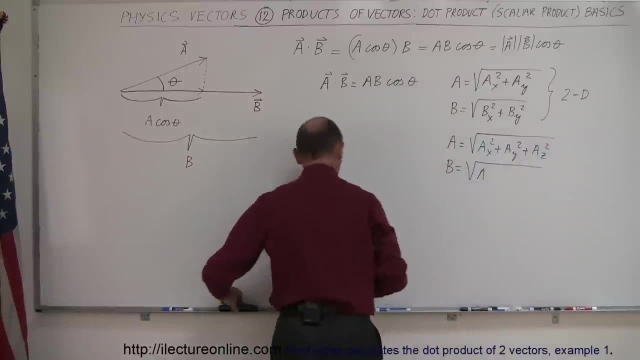 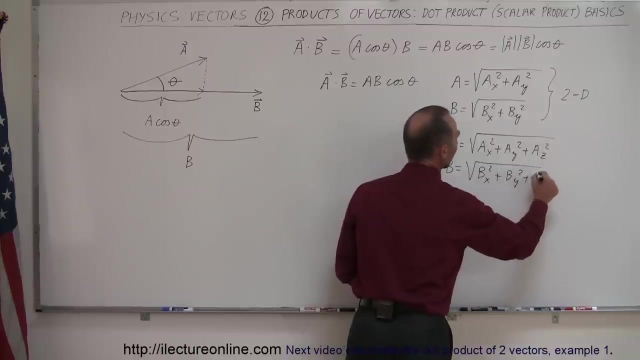 Plus the x component squared plus the y component squared plus the z component squared. Add it together and take the square root And of course for B that would be equal to A, not A, because I'm talking about the B vector. So in this case it would be B sub x squared plus B sub y squared plus B sub z squared. 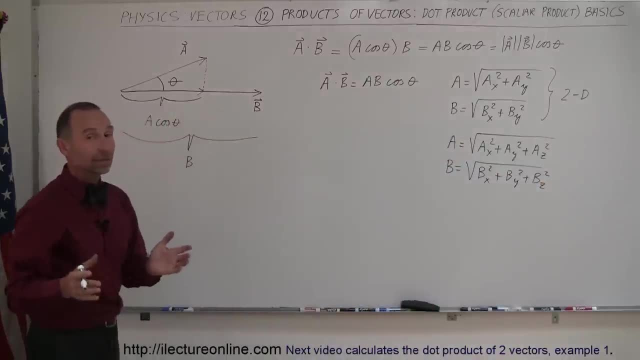 So that's how you find the magnitudes. So if you want to take a cross product, you take vector A and vector B. You find the x, y and z components, You square them, You add them together, So you find the magnitudes of the two vectors. 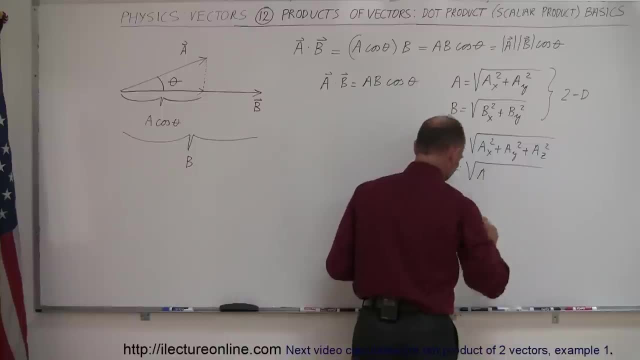 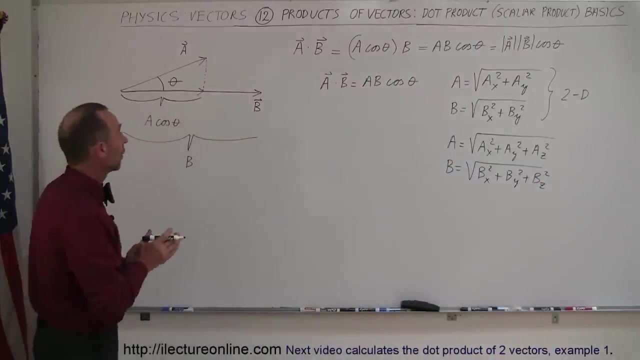 and of course for b that would be equal to a up, not a, because i'm talking about the b vector. so in this case would be b sub x squared plus b sub y squared, plus b sub z squared. so that's how you find the magnitudes. so if you want to take a cross product, you take vector a and vector b. 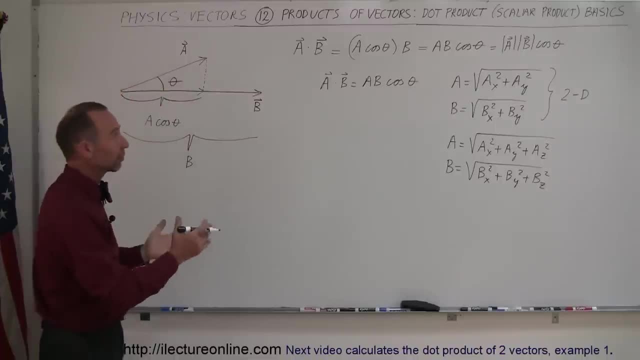 you find the x, y and z components, you square them, you add them together. take the square root so you find the magnitudes of the two vectors. multiply that together times the cosine of the angle between them and notice what if the angle between them is zero? so what if you had vector a? 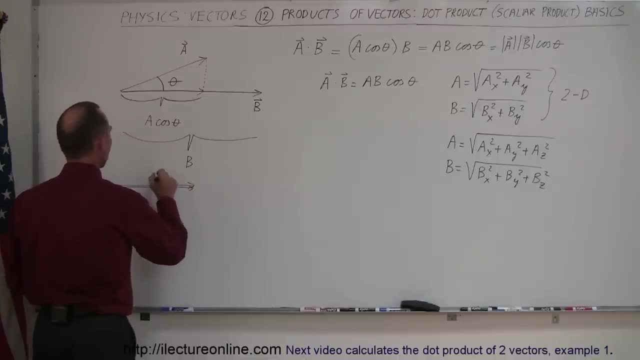 like this. and what if you had vector b like this: a and b, and of course they don't even have to be the same length- no vector b can be like this, of course- then the angle between them would be zero and the cosine of zero is one. so then, when you take the dot product, it's simply the magnitude. 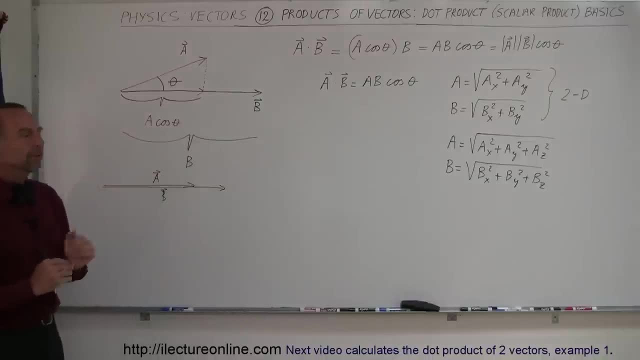 of a times the magnitude of b? you? what if they're perpendicular to each other? what if we had vector a like this? and what if i had vector b like this? what's the dot product? now? well notice, the projection of a on b would be zero length and the dot product of those two would be zero. and, of course, if you take 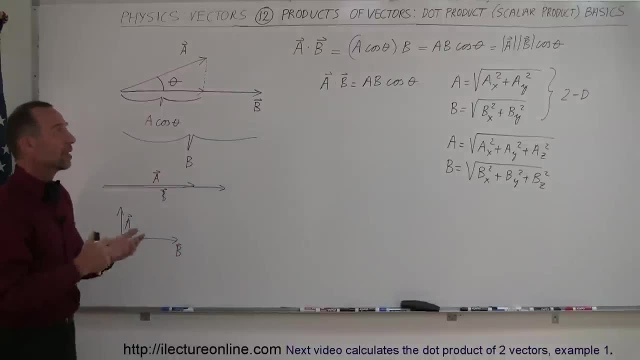 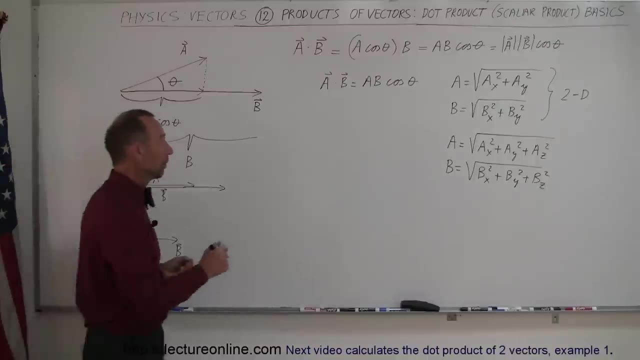 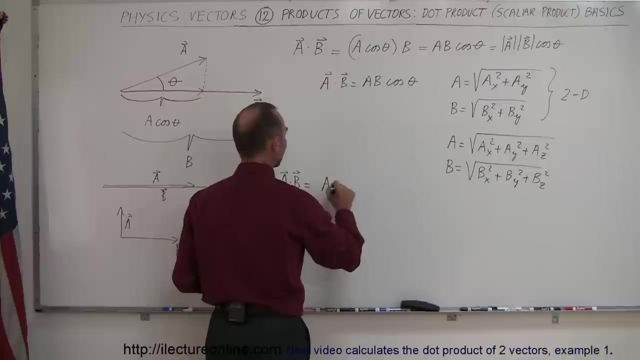 the cosine of 90 degrees. cosine of 90 degrees is zero and you get a zero result. there's one more way in which we can find the dot product of two vectors. it turns out that a dot b can also be found by saying that it's a product of the x components plus the product of the y components. 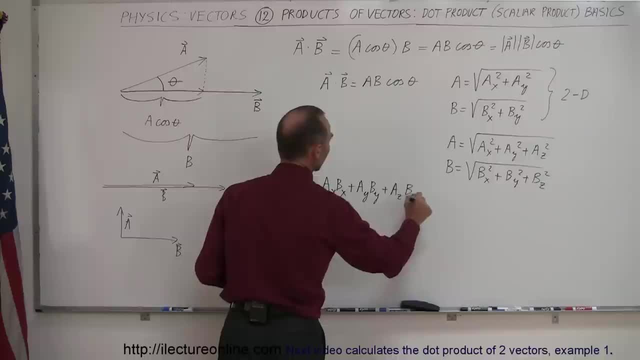 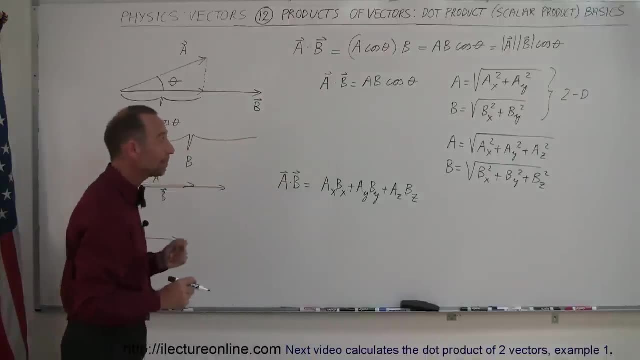 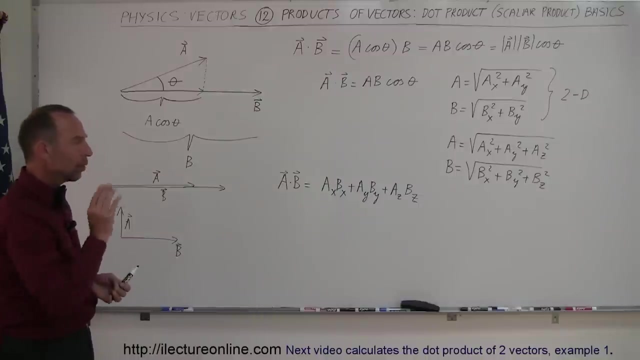 plus the product of the z components. so notice it's ax times bx, ay times by, az times bz. these are the magnitudes of those, not the. the magnitudes, not the, the vectors. and also keep in mind that the, if they're pointing in a negative direction, you do have to take into. 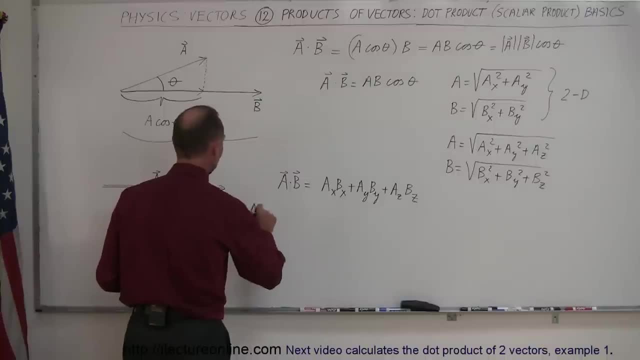 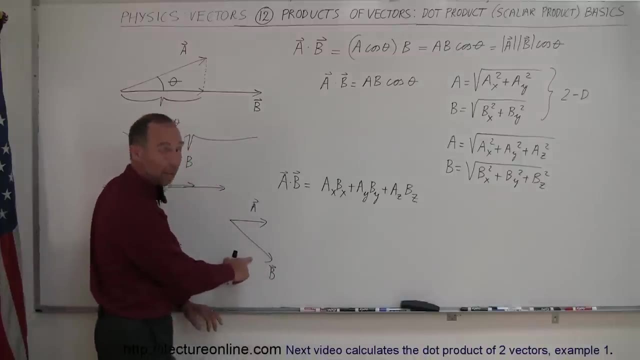 account the negative. For example, if I have a vector that looks like this, if this is the a vector, and I have another vector that is like this, this is the b vector. notice that this will have a negative y component, and so the 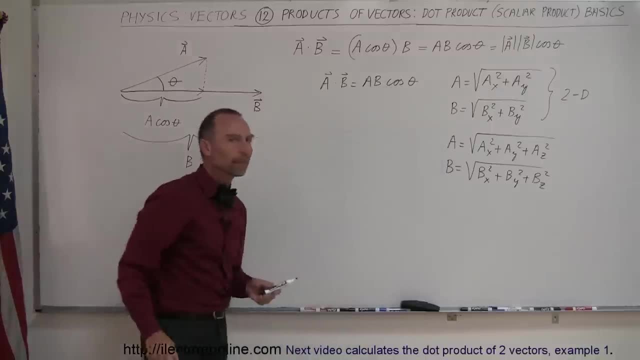 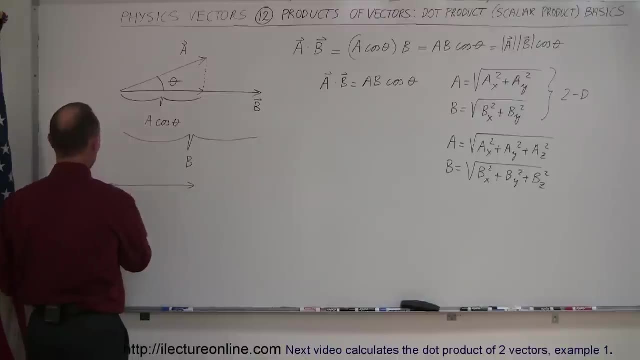 Multiply that together times the cosine of the angle between them And notice what if the angle between them is zero. So what if you had vector A like this, And what if you had vector B like this: A and B, And of course they don't even have to be the same length. 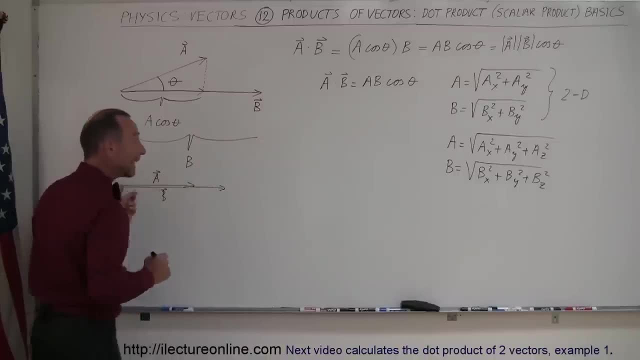 No vector B can be like this, Of course, then the angle between them would be zero And the cosine of zero is one. So then when you take the dot product, it's simply the magnitude of A times the magnitude of B. What if they're perpendicular to each other? 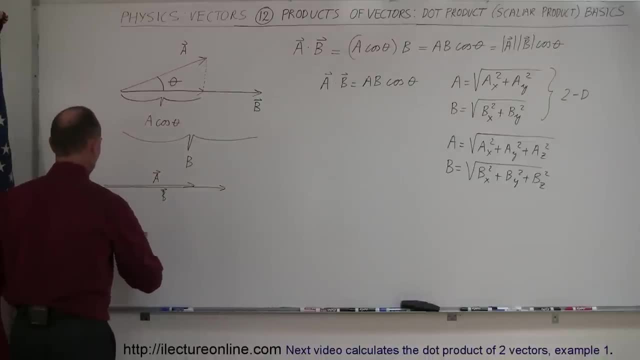 What if we had vector A like this, And what if we had vector B like this? What's the dot product now? Well notice, the projection of A on B would be zero length And the dot product of those two would be zero. And of course, if you take the cosine of 90 degrees, 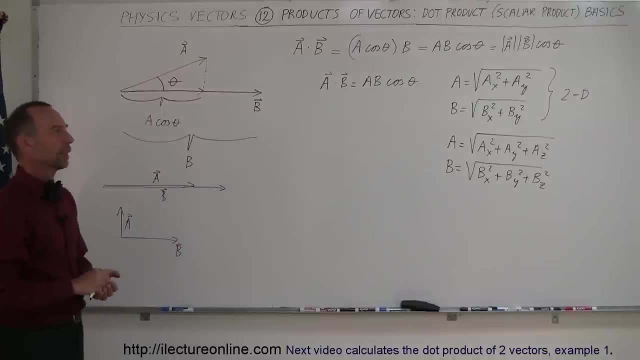 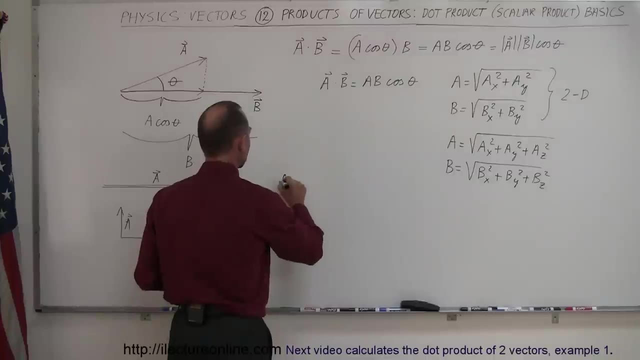 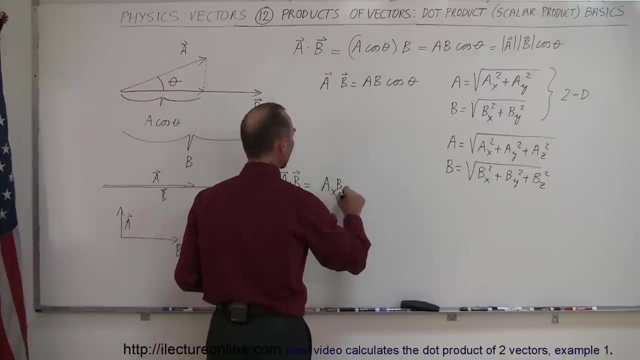 The cosine of 90 degrees is zero And you get a zero result. There's one more way in which we can find the dot product of two vectors. It turns out that A dot B Can also be found by saying that it's the product of the X components. 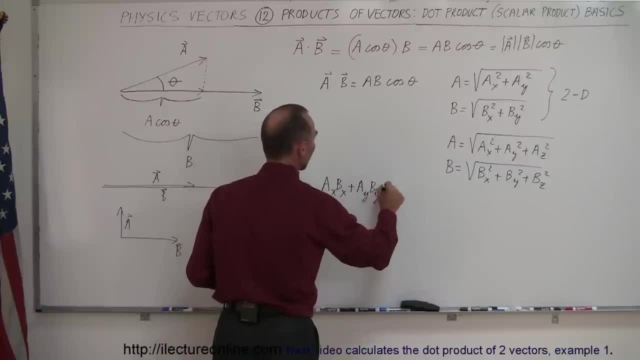 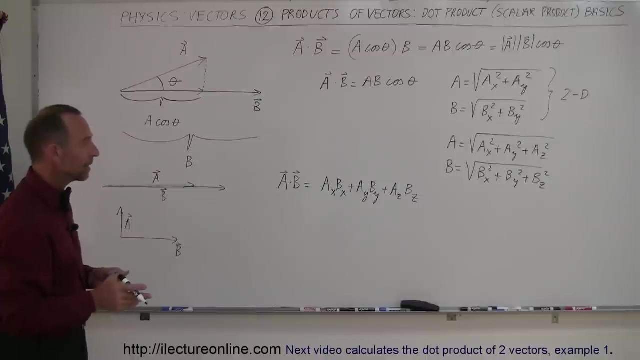 Plus the product of the Y components Plus the product of the Z components. So notice it's AX times BX, AY times BY AZ times BZ. These are the magnitudes of those, Not the. the magnitudes, Not the vectors. 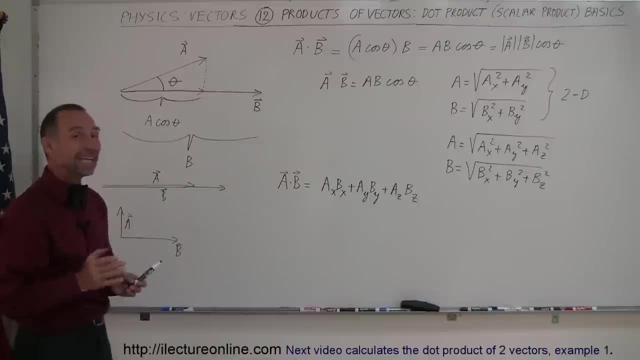 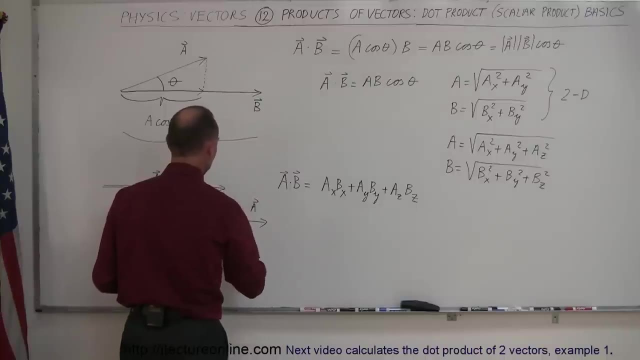 And also keep in mind That if they're pointing in a negative direction, You do have to take into account the negative. For example, If I have a vector that looks like this, If this is the A vector And I have another vector that is like this: 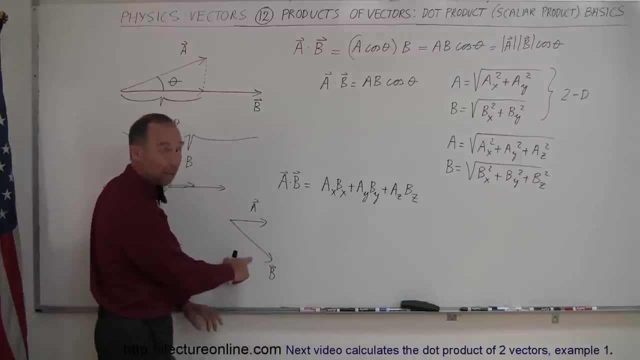 This is the B vector. Notice that this will have a negative Y component, And so the Y component would have to be negative, And if there's no Z components, Then of course Z simply would go to zero. So that's how we find the cross product. 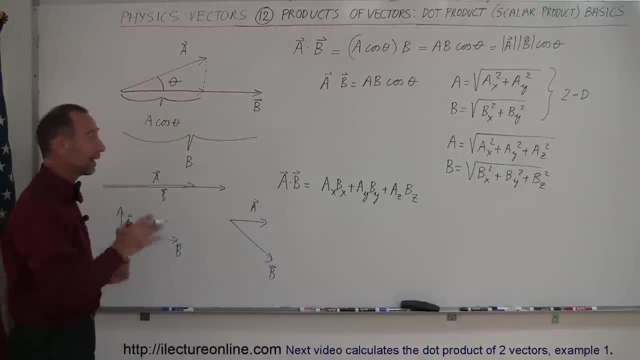 Now, of course, You probably would like to see some examples, So in our next video We'll do some examples Of how to find dot products, Of vectors.